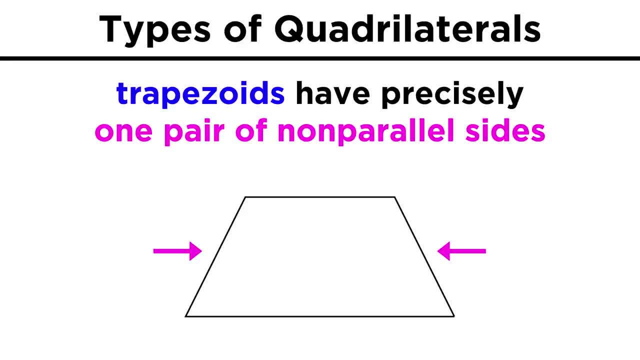 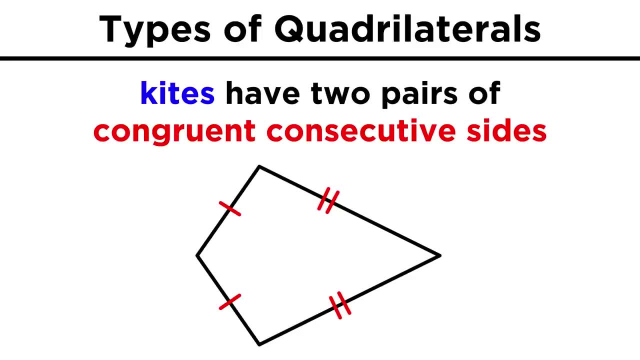 The other pair of sides must not be parallel, which can produce a variety of different trapezoids. A kite is a quadrilateral that has two pairs of congruent, consecutive sides. That means these two are the same length and these two are the same length. 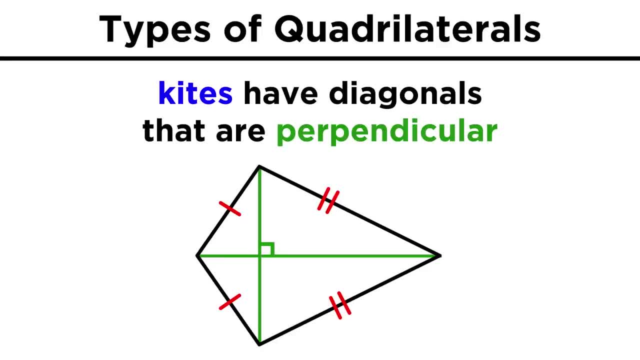 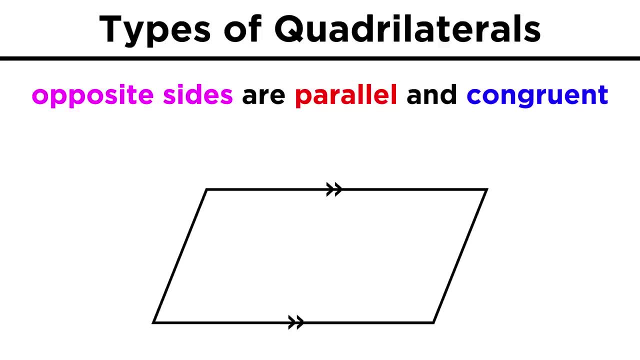 Kites have diagonals that are perpendicular. In this other quadrilateral, these opposite sides are parallel and of equal length or congruent, and so are these two. Because of this, opposite angles are also congruent. Any quadrilateral that meets these constraints is called a parallelogram. 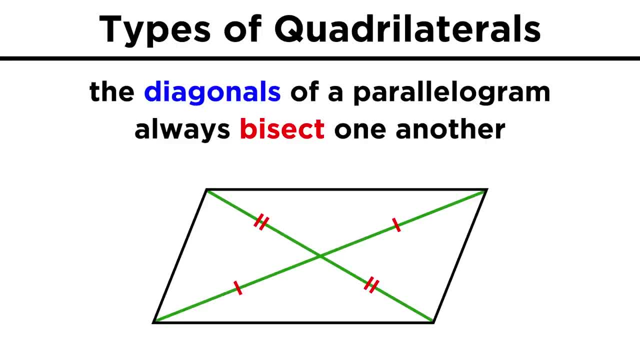 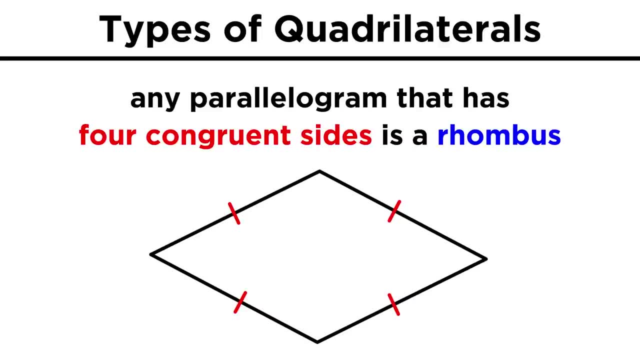 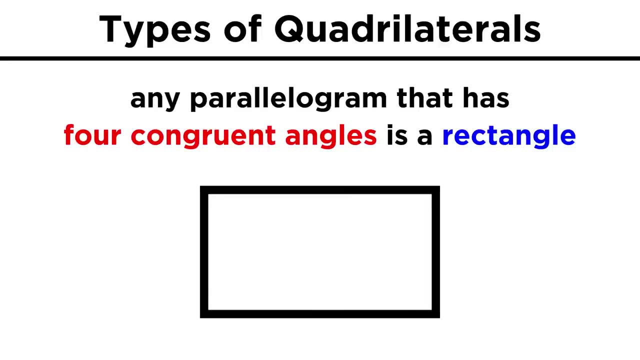 The diagonals of a parallelogram always bisect one another. Now, from here we can narrow things down further. Any parallelogram that has four congruent sides is called a rhombus. Any parallelogram that has four congruent angles, and therefore four right angles, is. 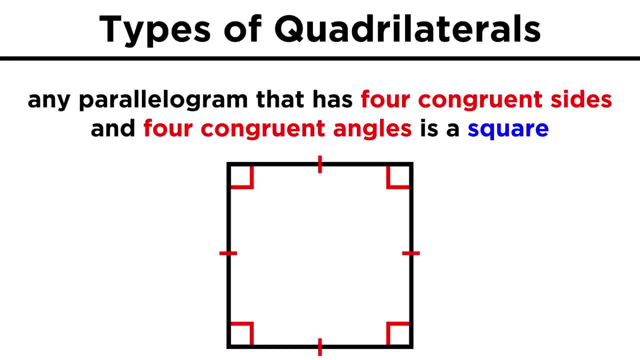 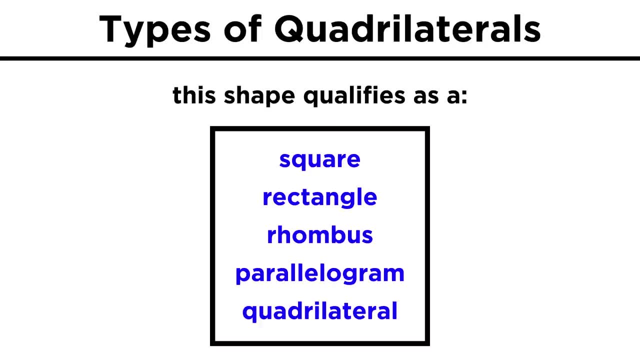 a rectangle. And, lastly, any parallelogram that has four congruent sides and four right angles is a square. Therefore, a square qualifies as a rectangle, rhombus, parallelogram and square In this diagram, and quadrilateral it is just a specific subset of these different shapes. 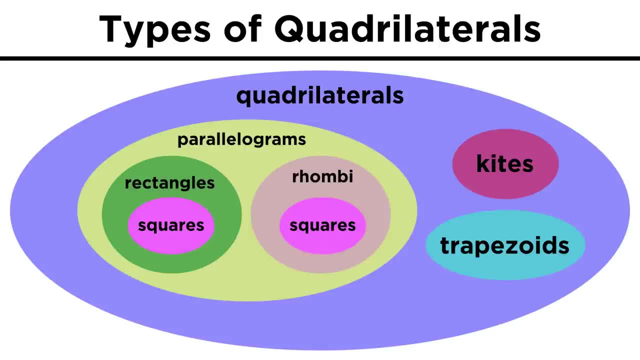 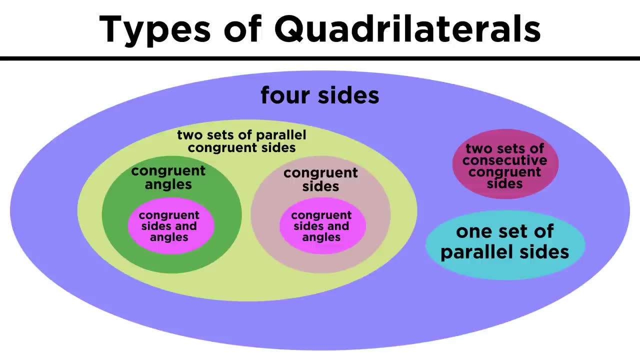 which we can see in this diagram, where different bubbles represent different shapes. Squares sit all the way in the middle, which demonstrates how they also qualify as some of the other shapes that have fewer constraints. So we can think of each new constraint as generating a new and more specific type of 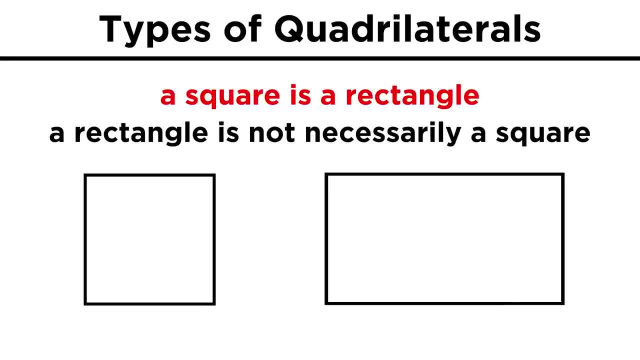 quadrilateral. This is what we mean when we say that a square is a rectangle, but a rectangle is not necessarily a square. Any square must have four right angles, so it is a rectangle, but it must also have four equal sides, and not all rectangles have four equal sides, so most rectangles are not squares. 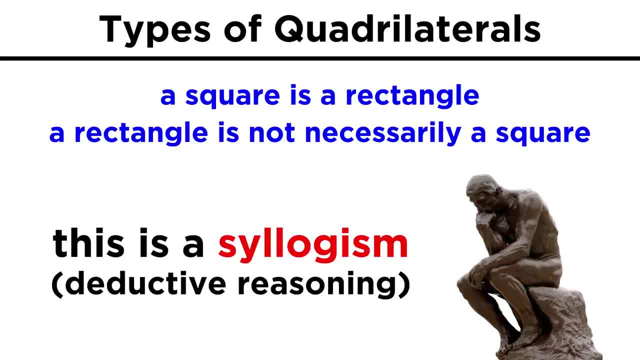 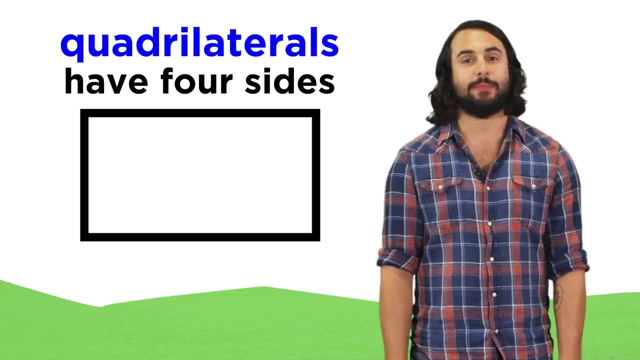 This is a syllogism, a form of deductive reasoning that we can use in everyday arguments, but we won't get into logic and philosophy here. So let's get started. Now that we know the various quadrilaterals, what about shapes with more than four sides? 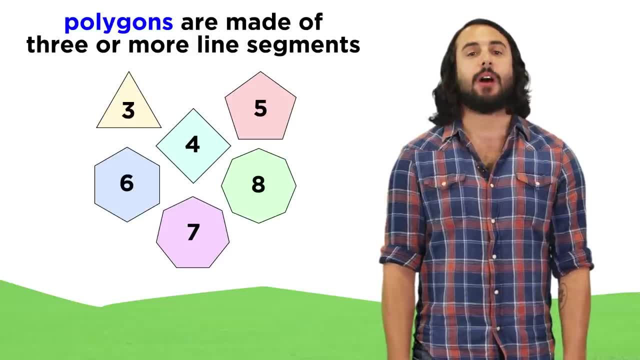 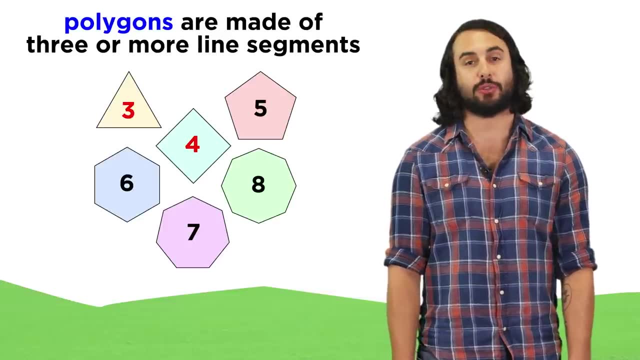 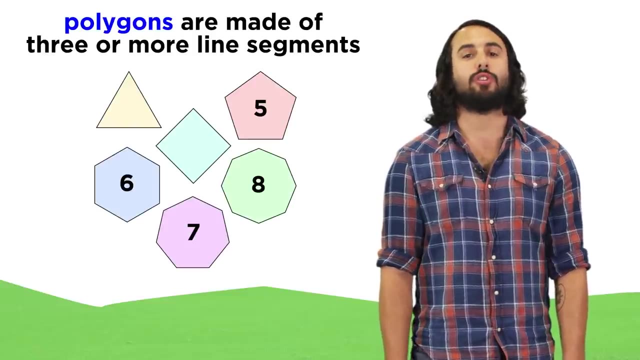 These are called polygons. To be specific, a polygon is any shape formed from three or more line segments. so triangles and quadrilaterals are technically polygons, But since we have specific names for those, we usually only use the word polygon to refer to shapes with five sides or more. 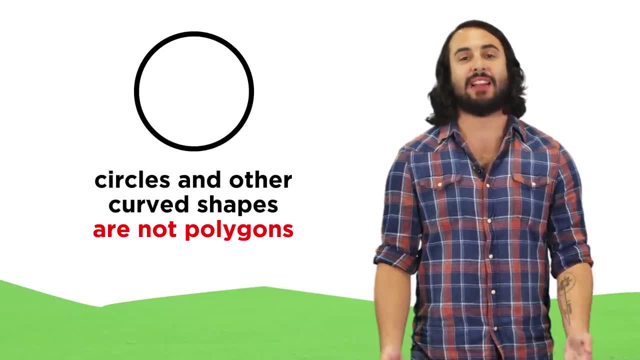 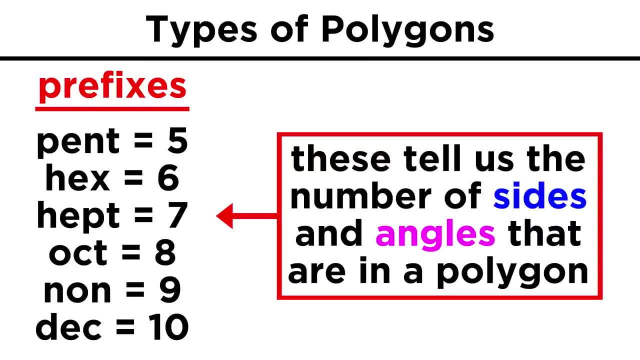 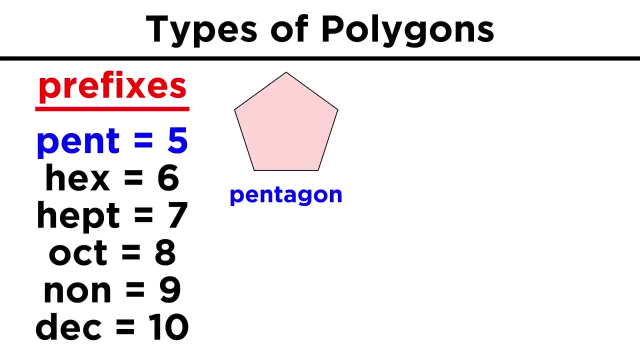 We must understand that only shapes with straight lines for sides count as polygons. so circles are not polygons. We have prefixes that indicate how many sides and therefore also how many angles are in a polygon. Starting with five sides, we can have pentagons, hexagons, heptagons, octagons, nonagons and 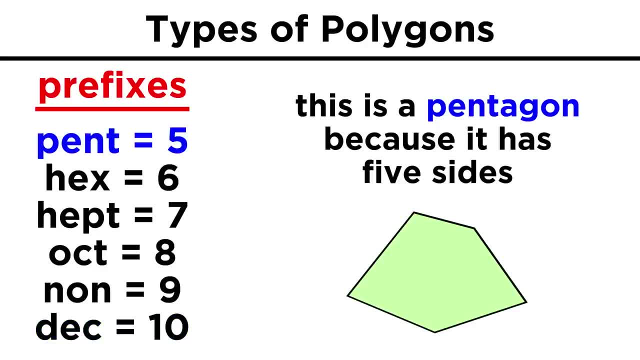 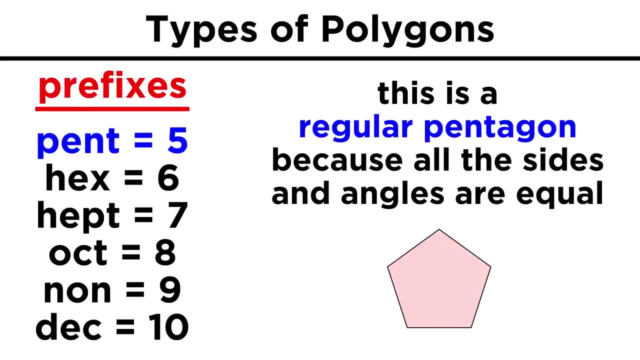 decagons To qualify as these shapes, they simply have to have these numbers of sides, which can be of any length and form any angles with one another. If a polygon has all of its sides and angles equal to one another, then it is a regular. 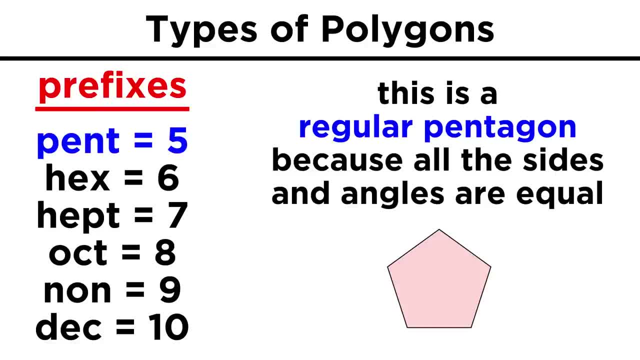 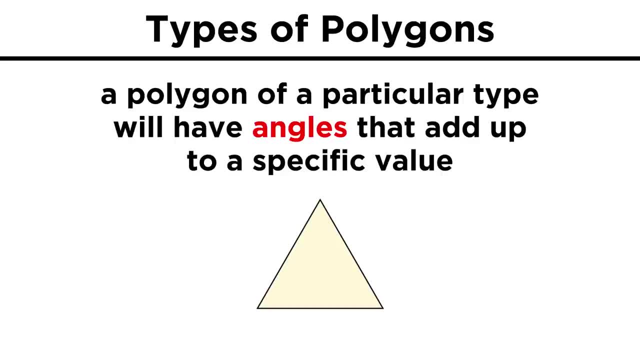 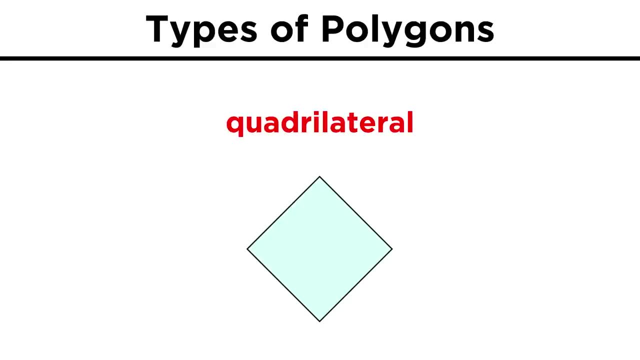 polygon, and these are the shapes that are most familiar to us. like the regular octagonal stop sign. Each shape will have its angles add up to a specific number. As we said, the angles of a triangle add up to 180.. A quadrilateral can be cut up into two triangles, so two times 180 means that the angles of 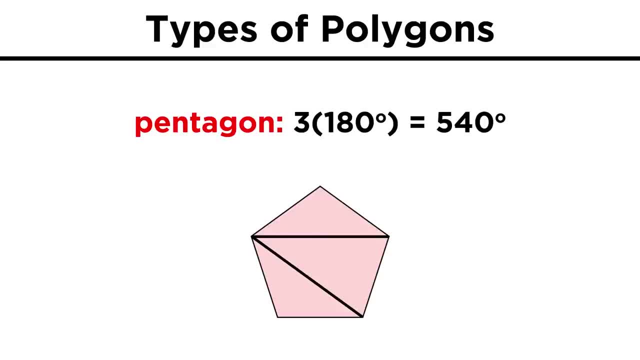 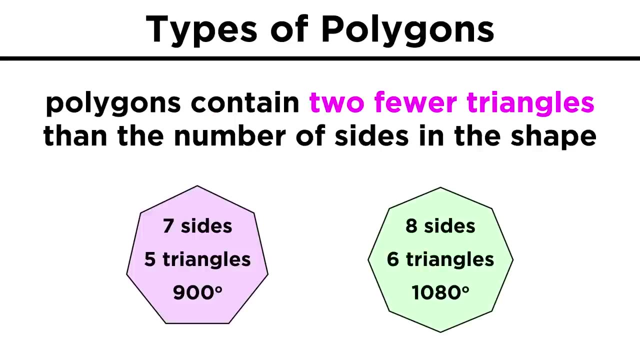 a quadrilateral will add up to 360.. A pentagon can be split up into three triangles, so its angles add up to 540.. A hexagon can be split up into four triangles, so its angles add up to 720.. We could go on and on in this fashion. 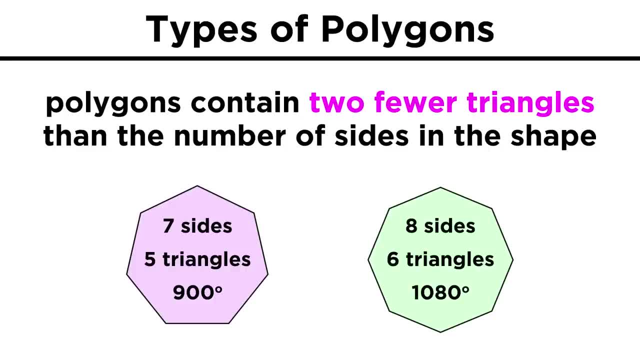 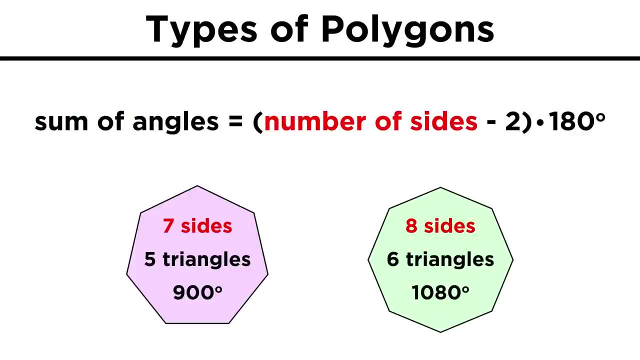 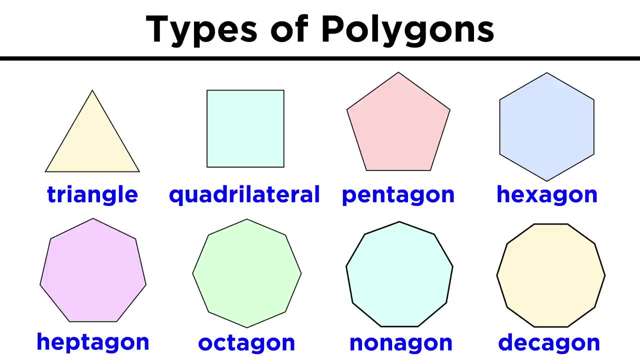 And every shape will contain a number of triangles, that is, two less than its number of sides. So to find out what the angles of a polygon add up to, take the number of sides it has, subtract two and multiply by 180.. Now that we know about a variety of shapes, let's check comprehension.